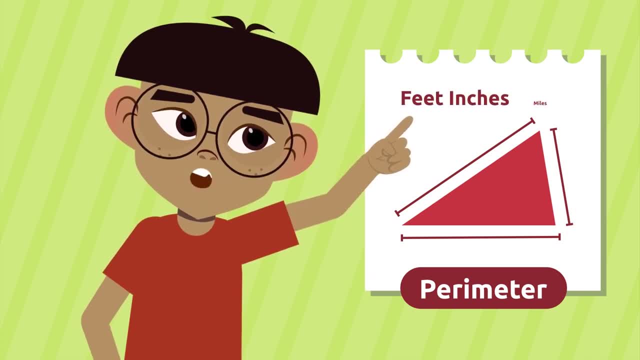 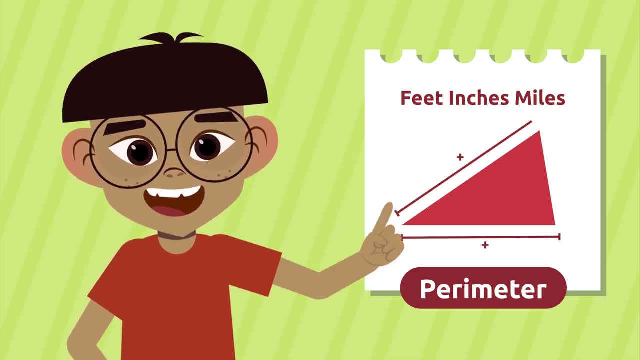 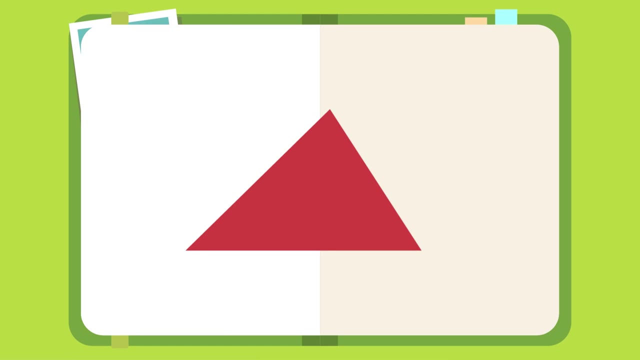 of its area. That's why it's measured in feet, inches, miles or other measuring units. To find the perimeter of a figure, we should add the lengths of each one of its sides. Let's look at an example. This triangle has three sides that measure 12,, 14, and 10.. To 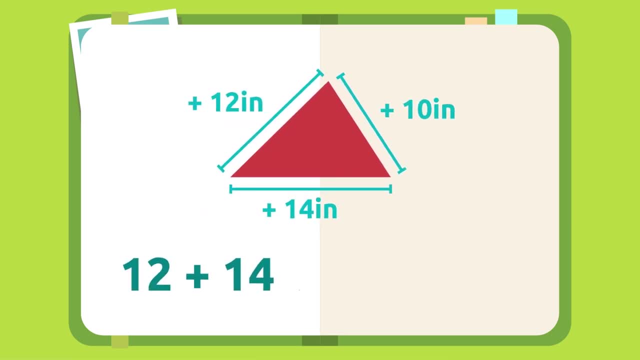 find its perimeter, we should add 12 plus 14 plus 10, which equals 36 inches- Awesome. This triangle has a perimeter of 12 plus 14 plus 10, which equals 36 inches- Awesome. This square has four equal sides. Each side measures 20 feet. To find its perimeter. 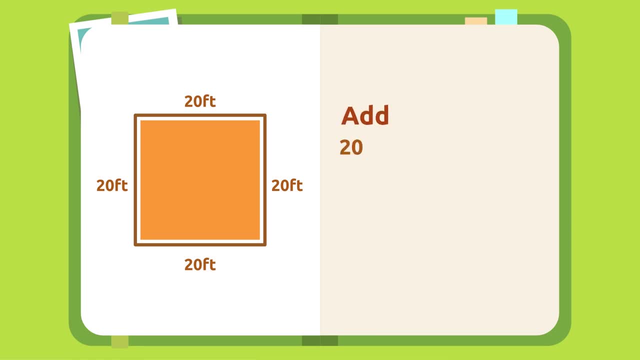 we can use two strategies: Add 20 plus 20 plus 20 plus 20, equals 80.. Or multiply four sides by 20 feet. Exactly, This square has a perimeter of 80 feet. In architecture or construction, knowing the perimeter is very important to be able. 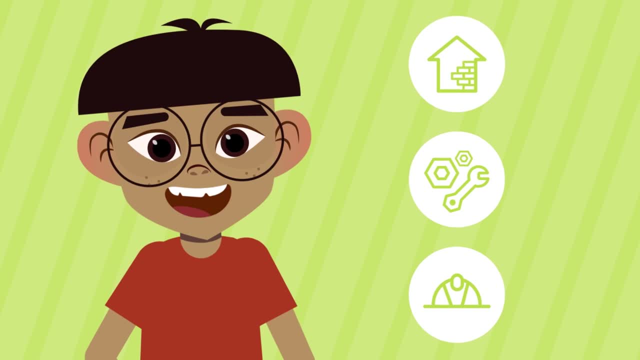 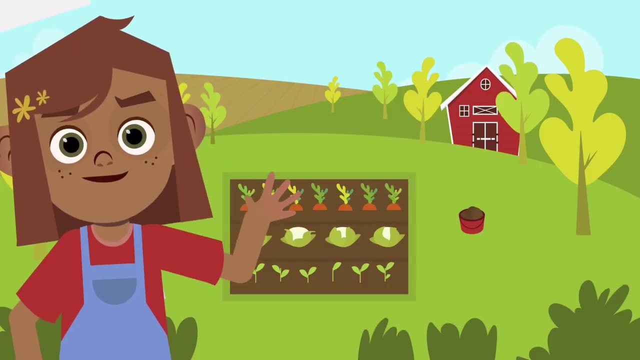 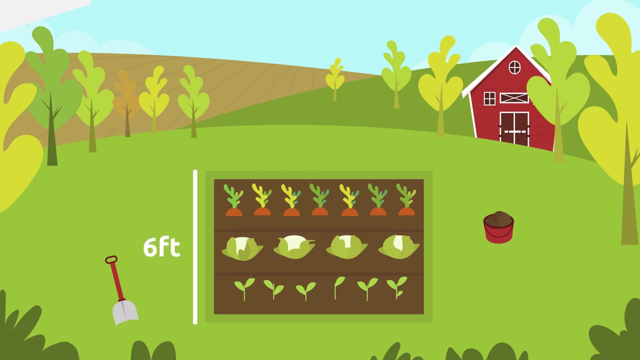 to calculate, among other things, the amount of material we're going to need. Now we're going to look at some examples. Anna wants to put a fence around the vegetable garden she built in her yard. The space has a rectangular shape and measures 6 feet wide and 10 feet. 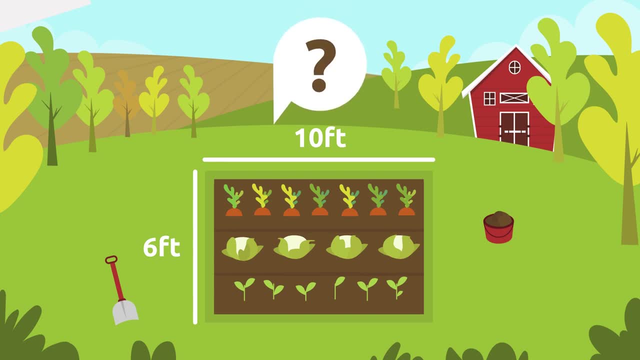 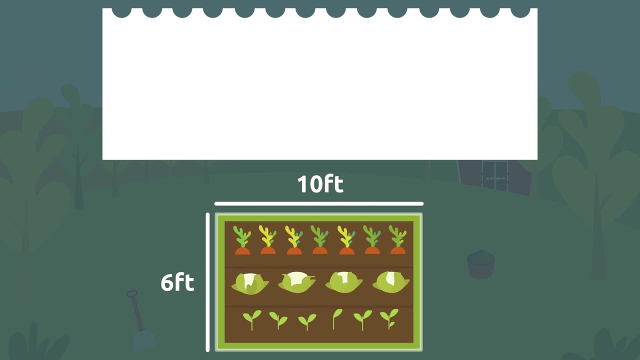 long? How many feet of fence material does she need to buy? To figure it out, we need to find the perimeter of this rectangle. We can use two strategies: Add 6 plus 6 plus 10 plus 10, which equals 32.. 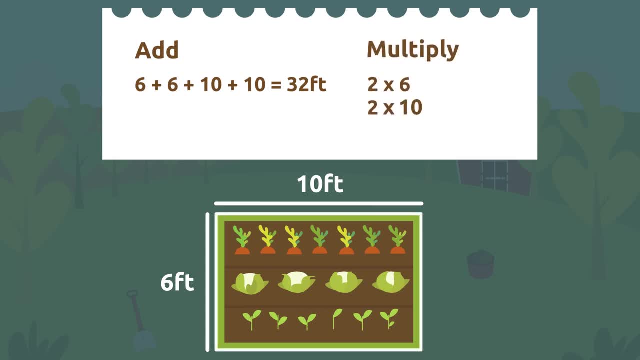 Or multiply two sides by 6 feet and two sides by 10 feet, Then we would have to add the results, That is to say 2 by 6,, which equals 12,, and 2 by 10, which equals 20.. 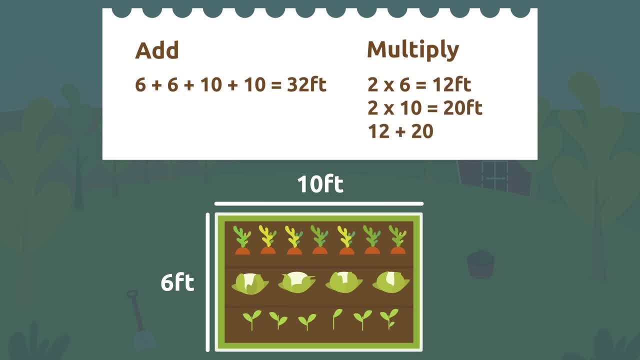 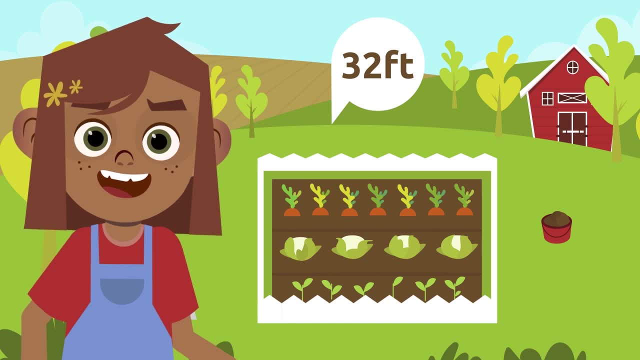 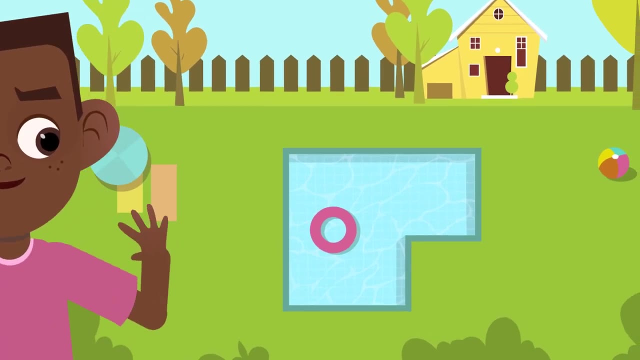 And now we add the results 12 plus 20, which equals 32.. Great Anna needs to buy 32 feet of fencing material to fence her vegetable garden. Let's look at another example. John wants to glue a white tape around his pool to separate it from the grass.